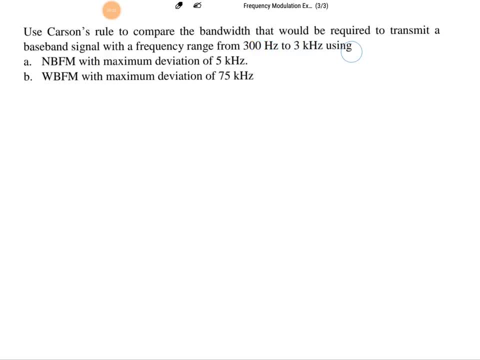 300 Hz to 3 kHz, using narrow-band frequency modulation with maximum deviation 5 kHz and using wide-band frequency modulation with frequency deviation 75 kHz. So for narrow-band frequency modulation here delta f max that is given and that is 5 kHz. 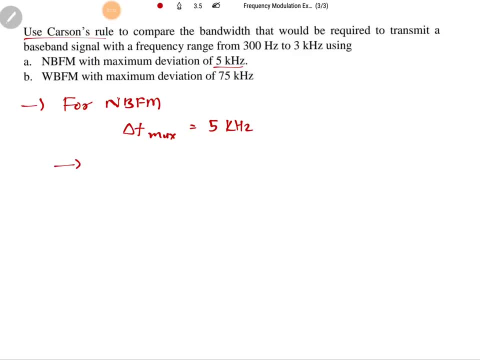 So as per Carnot's rule bandwidth of system that is given by 2 x fm max plus delta f max. so from that we can say: for narrow band frequency modulation here maximum frequency of modulating signal, that is 3 kilohertz. so 3 plus this is delta f max, that is 5 kilohertz. 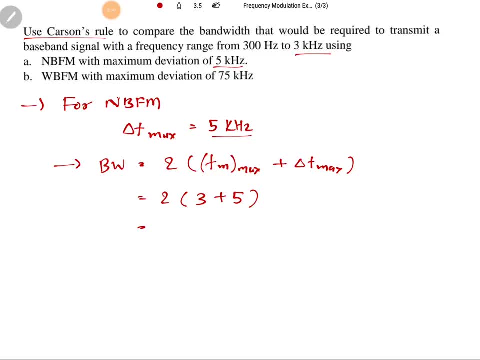 so this will be 8 into 2, this will be 8 into 2, so that will be 16 kilohertz. now for wideband frequency modulation. here delta maximum deviation is given, that is 75 kilohertz, so where we can apply carnos rule and based on that we can identify bandwidth. 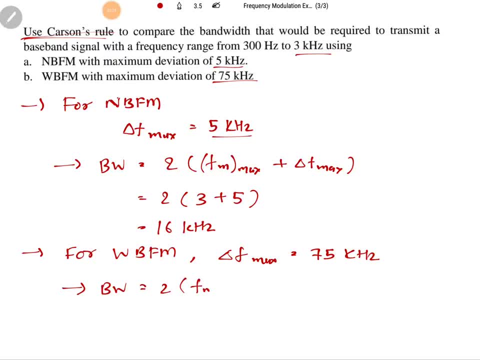 so that is 2 into FM max plus delta of max. so here this will be 2 into FM max. so that is 3 kilohertz maximum frequency of modulating signal plus Delta f max. that is given by 75 kilohertz, so 75 plus 3. 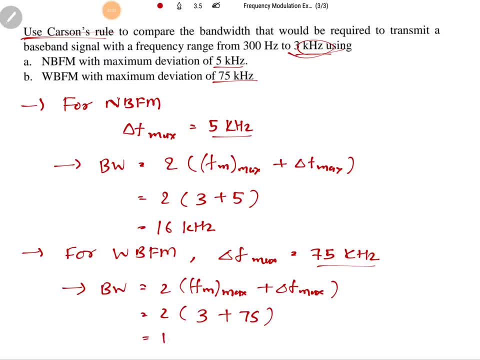 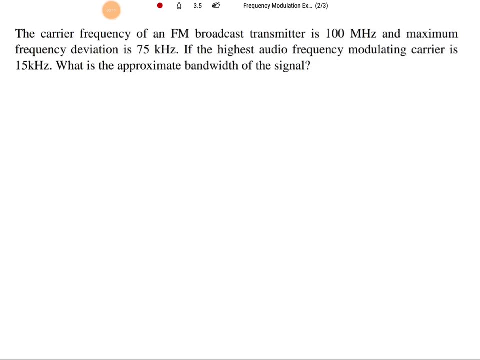 that is 75 plus 75 plus 75 tools, internet cell control. so latent 10 suis into 2, that will be 156 kilohertz. so that is how we can identify bandwidth using Carnot Carson rules. now let us solve next problem, and here the carrier. 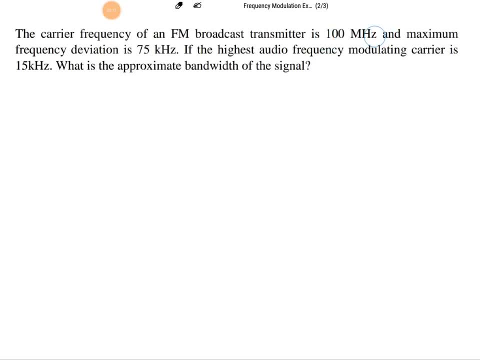 frequency of FM broadcast transmitter is 100 megahertz. that is given. so let us mention step by step: at C, that is 100 megahertz, maximum frequency deviation is given by 75 kilohertz. so Delta f max that is given by 75 kilohertz, if highest. 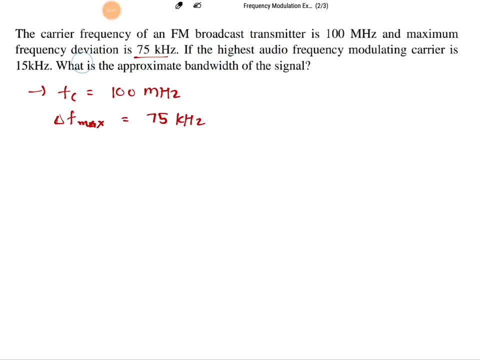 audio frequency of modulating carrier is given by, say, 15 kilohertz. So here, modulating frequency with highest value, that is given by 15 kilowatts, What is the approximate bandwidth of this given signal? Now, approximated bandwidth that we can easily calculate it by Carson's rules. 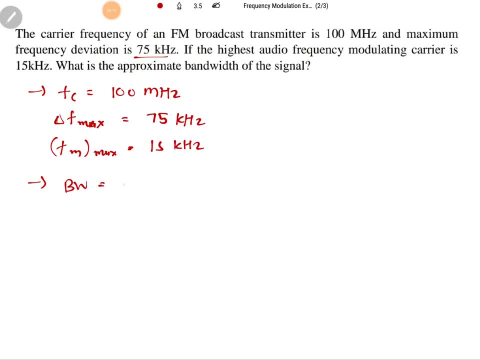 So that bandwidth by Carson's rules that is 2 into FM max plus maximum deviation. Now here all the values that is there with us, So that will be 2 into this FM max, that is 15 kilowatts, plus delta, F max, that is 75.. 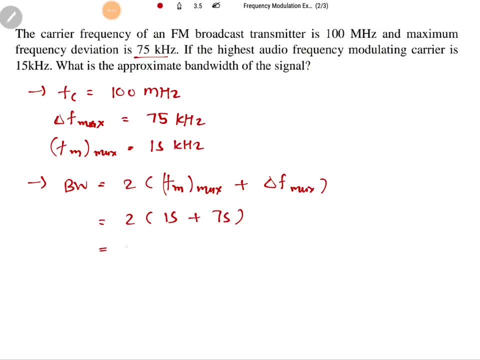 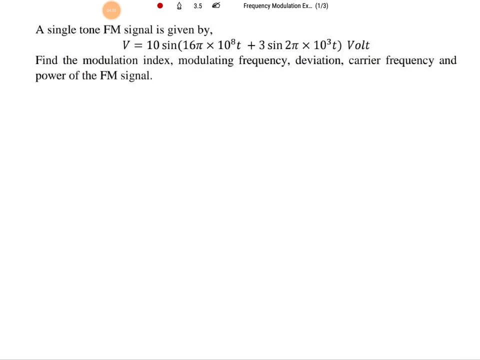 So 75 plus 15, that is 90 into 2.. So 90 into 2 is 180 kilowatts. So that is how we can identify bandwidth by using Carson's rules. Now let us solve next problem. Now see in this FM signal V that is given by 10 sine, 16 pi into 10, to the power 80.. 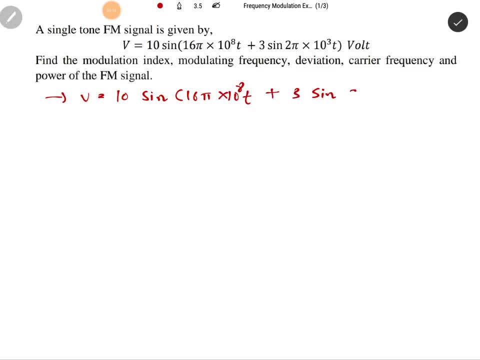 Plus 3 sine into 2, pi, into 10, to the power 3T In terms of voltage it is given. So we are delivered to calculate modulation index, modulating frequency, deviation, carrier frequency and power of FM signal. So to calculate that first we need to compare this equation with standard equation. 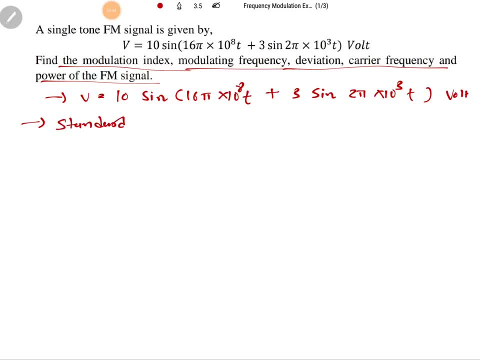 So Standard equation for FM that we know, that is V, is equals to EC sine omega CT, plus modulation index MF into sine of omega MT. So if we do this comparison we will be getting: EC is equals to 10 voltage, Omega C, that is equals to 16 into pi, into 10, to the power 8.. 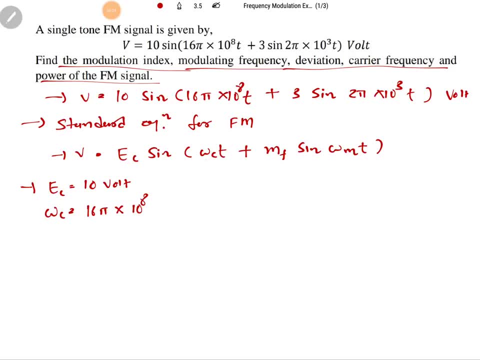 So 16 pi into 10 to the power 8, after comparison of this: 2. Then modulation index, MF, that is 3. Based on this comparison, And omega M, that is 2 pi into 10 to the power 3, that is how we can compare this to now, based on omega c. 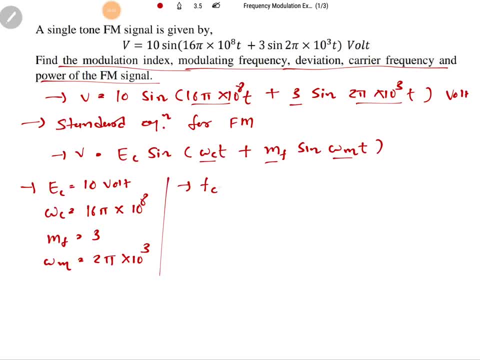 based on omega c. we can say fc, that is, omega c by 2 pi, so we'll be having 8. if you place this value- 16 pi- into 10- to the power, 8 divided by 2 pi, so that will be 8 into. 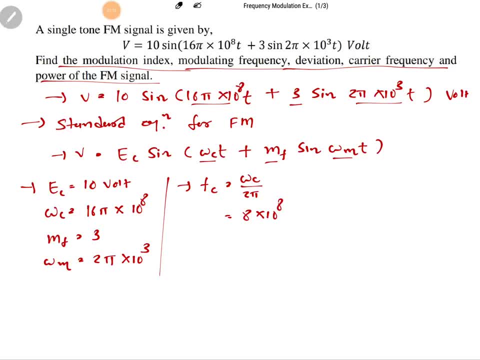 10 to the power 8 hertz and fm. that is omega m by 2 pi. so if you place that value, 2 pi will get cancelled and fm will be 10 to the power 3 Hertz. now modulation index is given, so modulation index that is useful to get that. 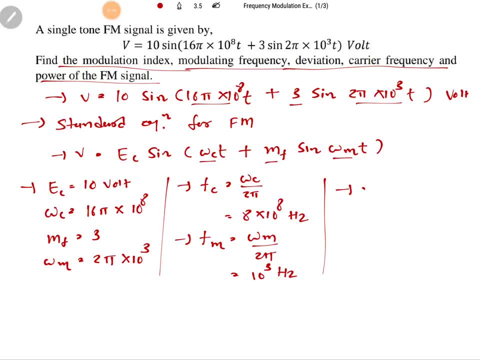 modulation index. that is useful to get that modulation index. that is useful to get that frequency deviation, see modulation index M F, that is deviation divided by maximum modulating frequency. so deviation that is M F into FM so we can say deviation that will be M F. that is what 3 and